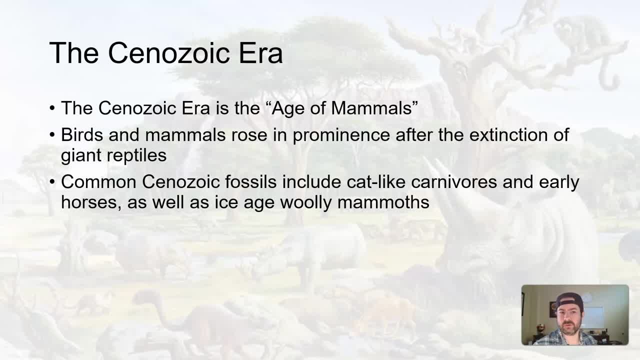 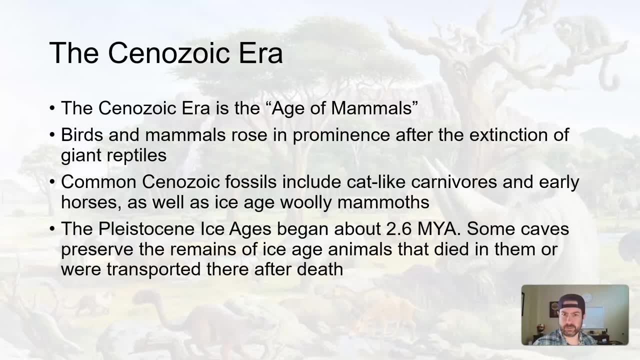 Some common fossils we find are cat-like carnivores, early horses, Ice Age woolly mammoths And then during the Pleistocene Ice Ages, about two and a half million years ago, some caves preserved Preserve the remains of Ice Age animals that either died in them or were transported there after death. They were washed in there after death. So there's a lot of fossils from the Cenozoic era and from the Ice Age, mostly because it's what happened most recently. 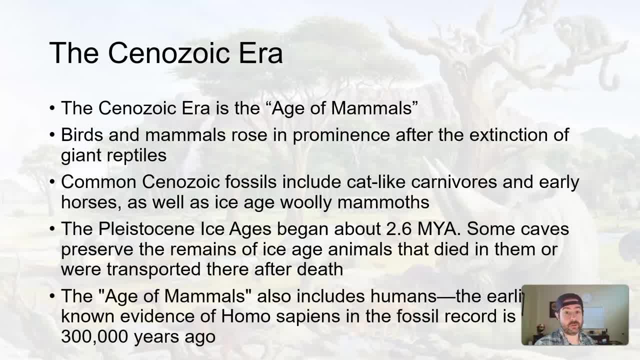 When talking about the Age of Mammals, we also have to talk about humans, which are mammals. the earliest known evidence of Homo sapiens, which is our species, In the fossil record, it's from about 300,000 years ago. 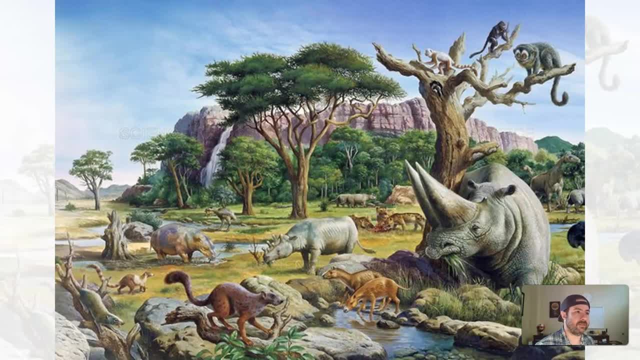 It's a little view of what Cenozoic life would have been like: Some early primates, small and evolving to larger mammals. Grasslands are developing. The Earth is, geologically speaking, weathering and erosion. Trees already existed. 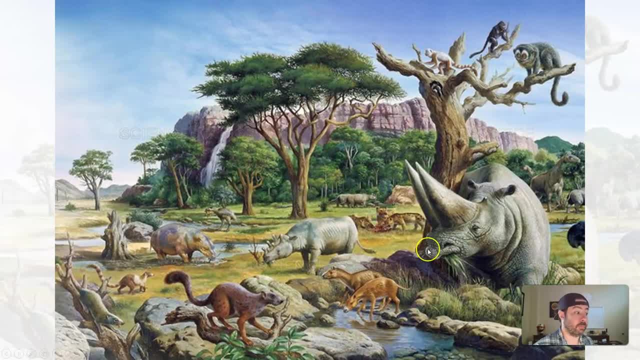 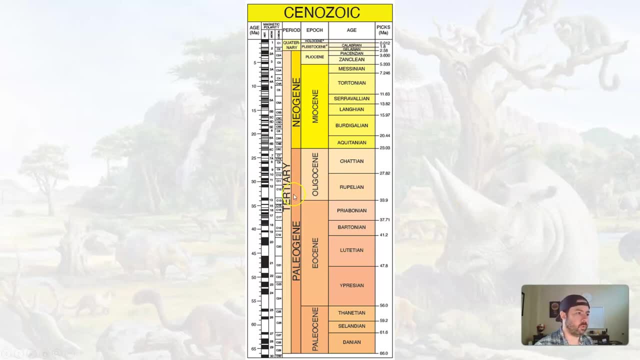 So mammals are really the things that and birds Are really the things that come to prominence during this time. Again, we'll break it down. This lecture is broken down into a few different sections: The Paleogene, Neogene and the Quaternary. 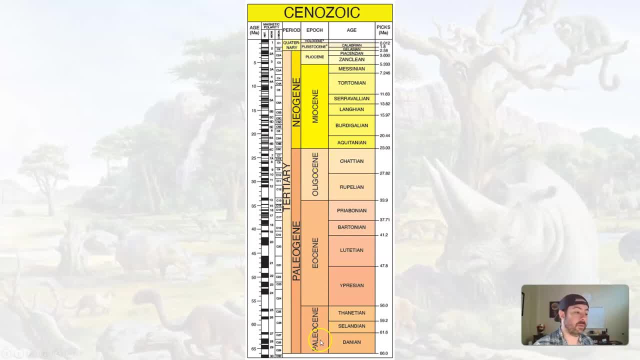 But during those we'll break it down further into epochs: The Paleocene, Eocene and the Legocene epoch during the Paleogene period, And the Miocene and Pliocene epoch of the Neogene period, And the Pleistocene and Holocene epoch of the Quaternary. 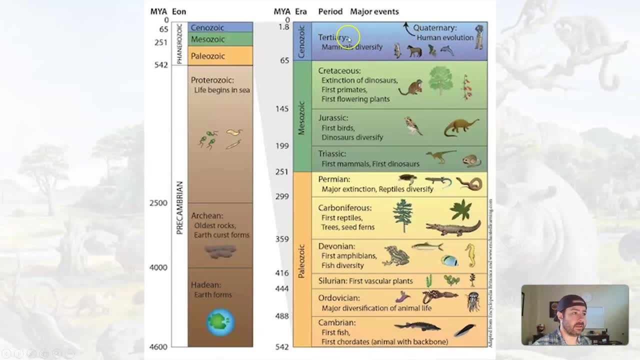 The Pleistocene and Holocene epoch of the Quaternary period. Again, really, mammals and bird mammals evolve, or I should say mammals evolve. Mammals existed back in the Mesozoic, but they diversify as well, as birds and humans evolved during this time as well. 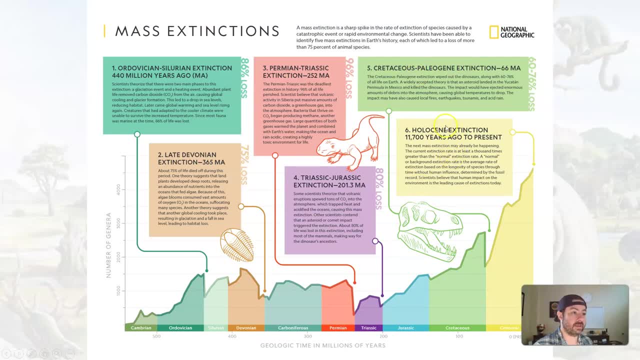 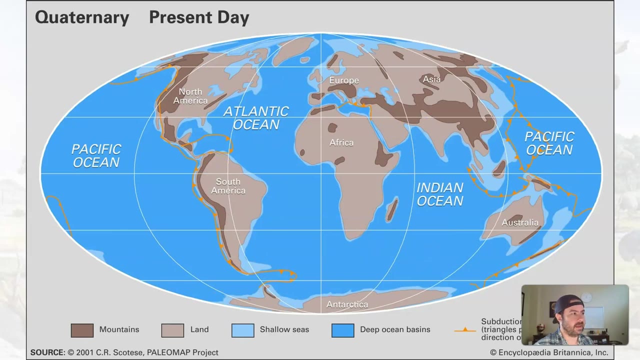 There was one extinction, or I should say not even one. there is an extinction- It's actually currently ongoing and we'll talk about that once we get there- Started off. this was the first extinction. The Cenozoic started off Earth looking like this and ended present-day what we now know. 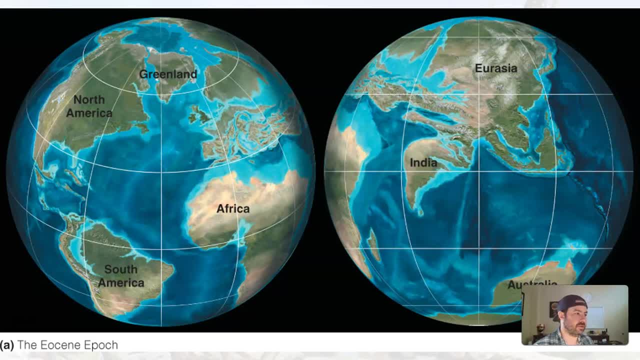 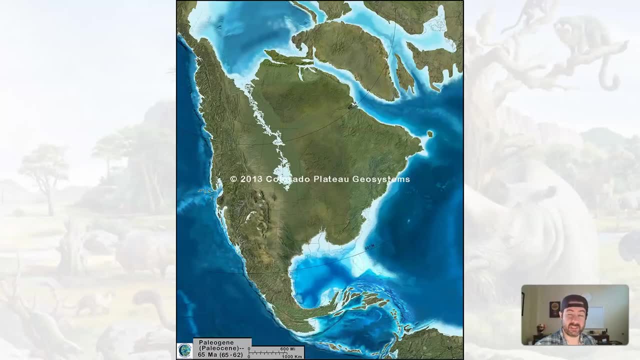 So Pangea- that further breakup of Pangea's things moving away until they get into present-day locations, How we started the Cenozoic and how we ended the Cenozoic- We talked a lot about that in Unit 13 of the Earth History. 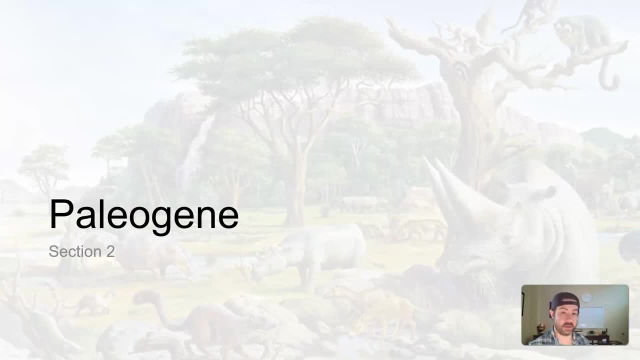 So let's go ahead and put this together. We'll pause there and when we come back let's jump into the life of the Paleogene. We'll see you back here in just a second. 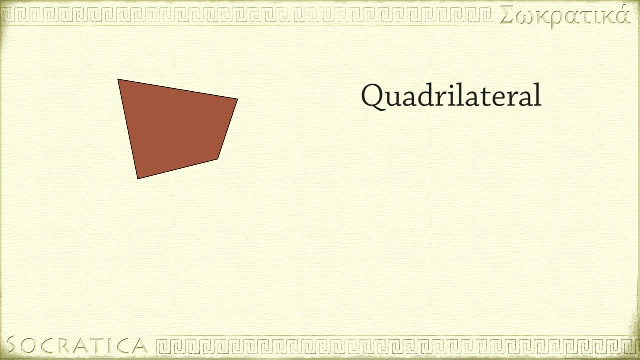 A four-sided polygon is called a quadrilateral. The word quadrilateral is a combination of quad, which means four, and lateral, which means side. Quadrilaterals are given specific names depending on whether there are parallel sides, equal angles or equal sides. 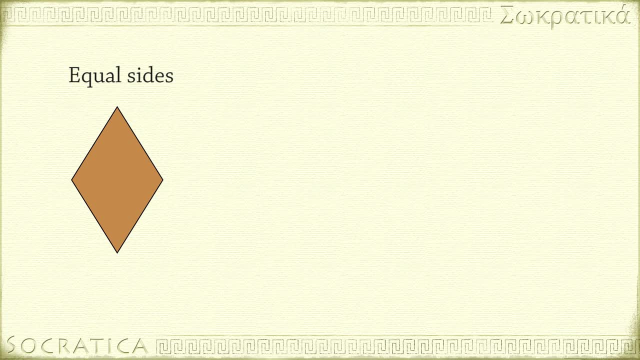 If all four sides are the same length, we call the shape a rhombus. When all four angles are the same, we call the shape a rectangle. In this case, all angles measure 90 degrees. All four angles are right angles. 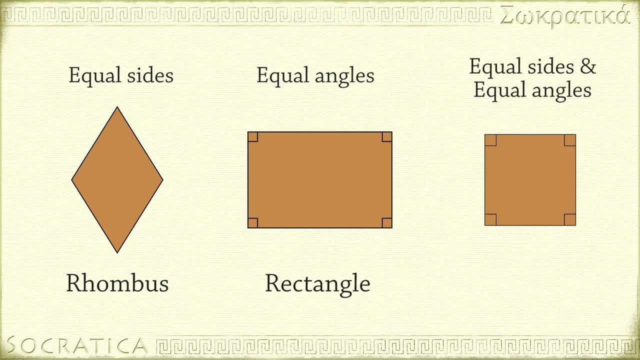 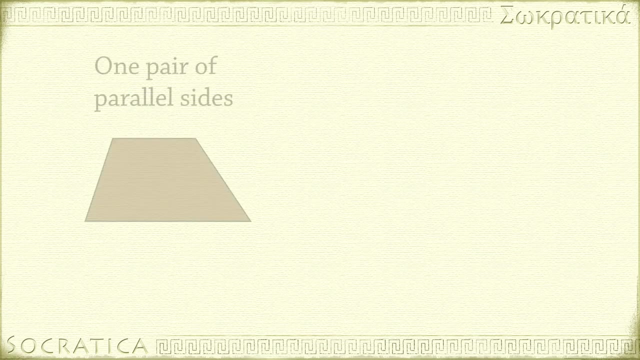 If all four sides are equal and all four angles are equal, the shape is called a square. In addition to classifying quadrilaterals by their sides and angles, there are also specific names depending on whether or not opposite sides are parallel. If one pair of sides are parallel, 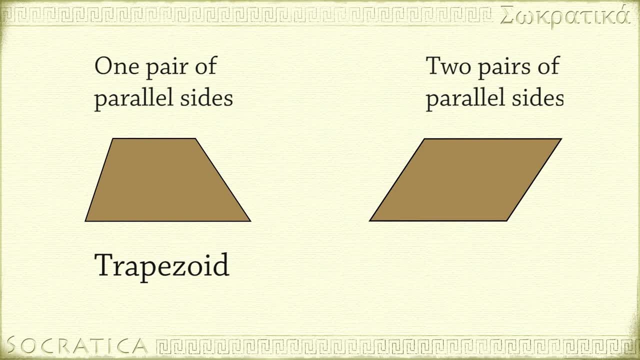 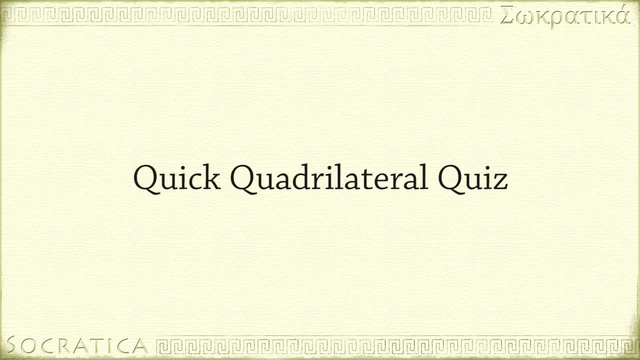 the shape is called a trapezoid. When both pairs of sides are parallel, the shape is called a parallelogram. Try and identify the following quadrilaterals. The rule of thumb is to use the most specific name when describing a shape. 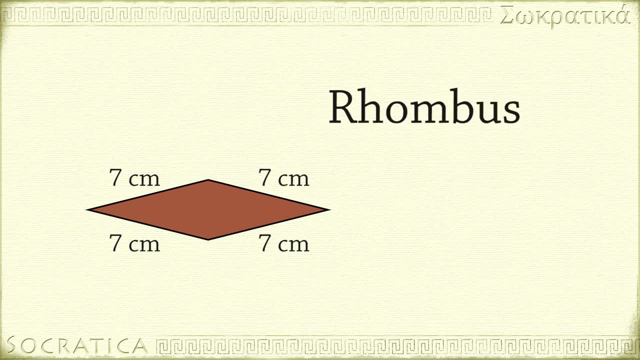 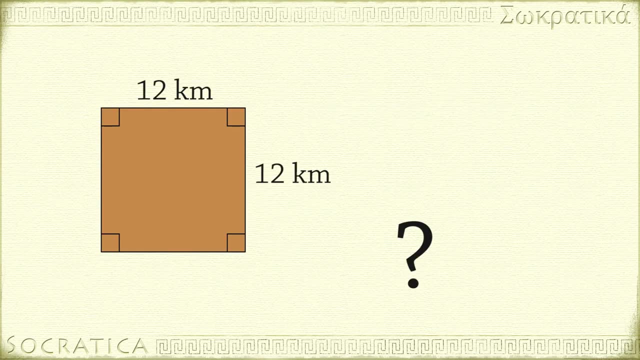 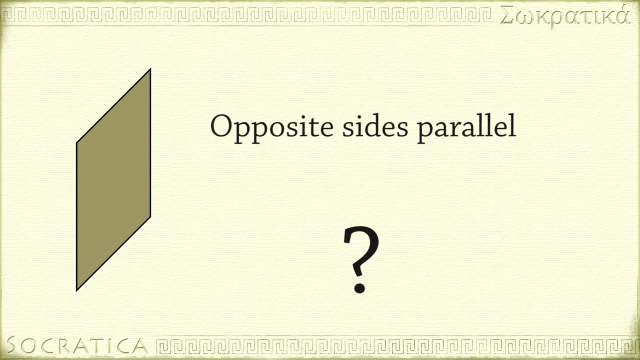 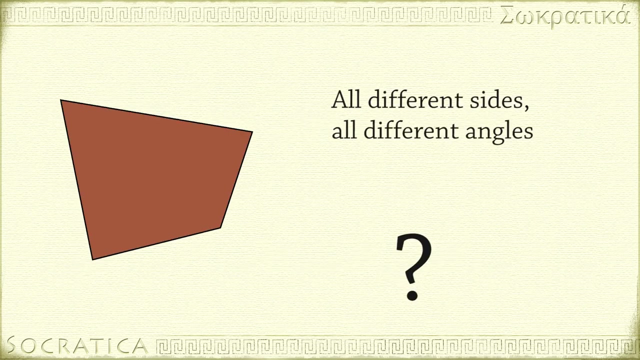 For a good majority of quadrilaterals the tip should be 70 degrees, which is the center point. For 5 makes of that 0 degrees. it is novel. 1. The center point is always 100 degrees. Suppose that you place a half- WOW.